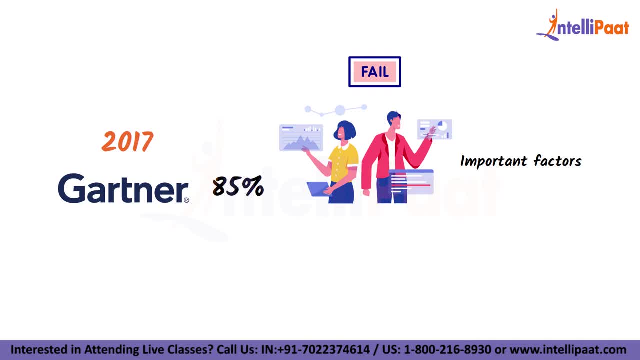 data projects failed. One of the most important factors leading to this was the available data infrastructure was not reliable enough to make business decisions. According to the CTO of IBM, in 2019, 87% of data science projects could never make it into production. Why is that, If data is? 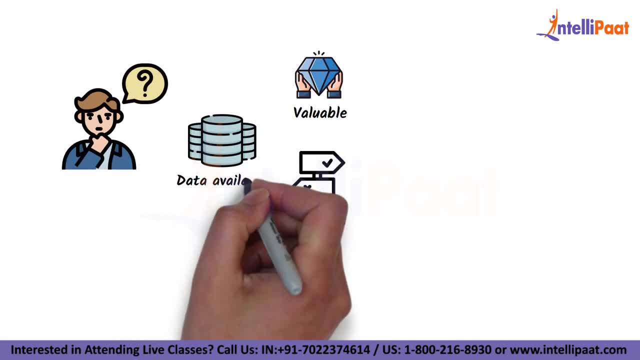 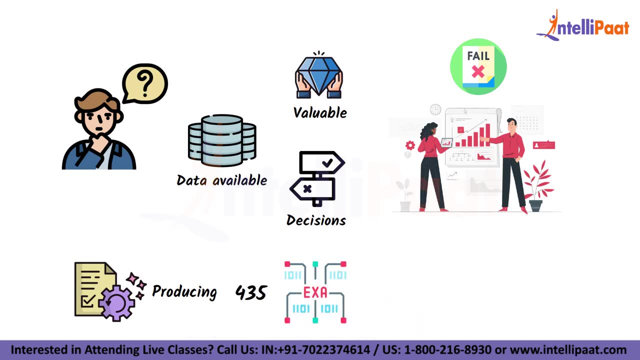 so valuable and most decisions can be made using the data available, then why were so many data projects failing? Well, we are moving towards a world where we will be producing 435 exabytes of data per day. To put that in perspective, that's one followed by 18 zero bytes worth. 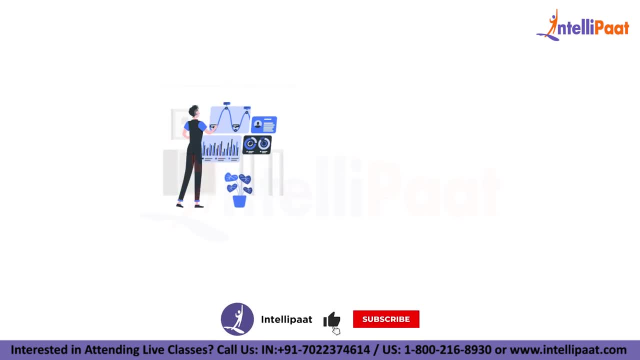 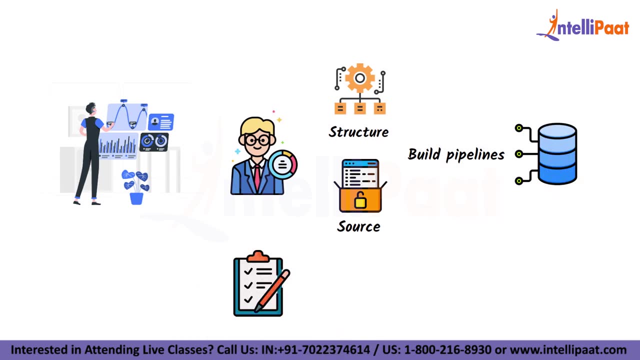 of data. This is where data engineers come into picture. Earlier data scientists were expected to structure, source and build pipelines for data. These tasks were often out of data scientists' scope of work or their skill set. The result was that data modeling would not be done correctly There. 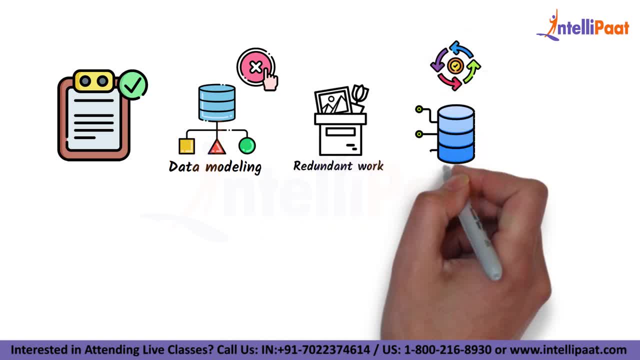 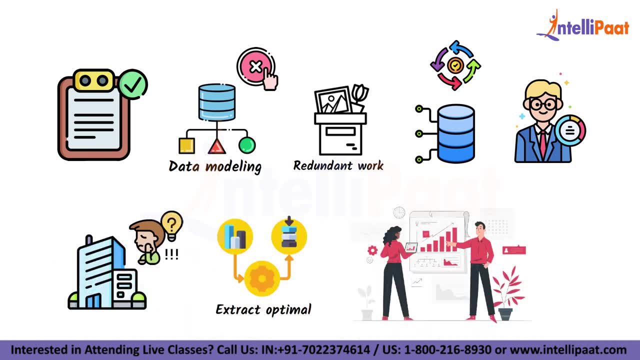 would be a redundant work and inconsistency in the use of data among data scientists. These kind of issues prevented companies from being able to extract optimal value from their data projects, so they failed. Eventually, more and more organizations began to realize the need of professionals who can. 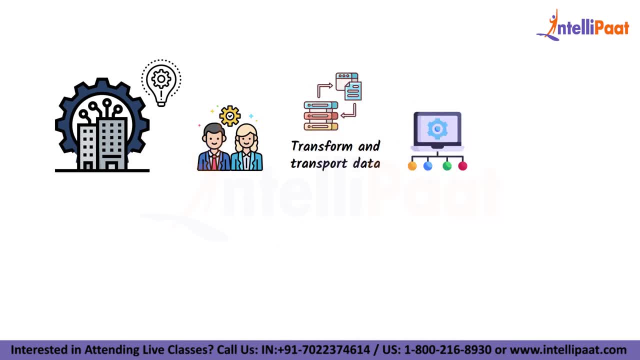 transform and transport data in such a way that, by the time, it reaches an end user, like data scientists, they are in highly usable format. Data pipelines are created by data engineers and they are used to build a warehouse of data collected from different sources and used across the entire. 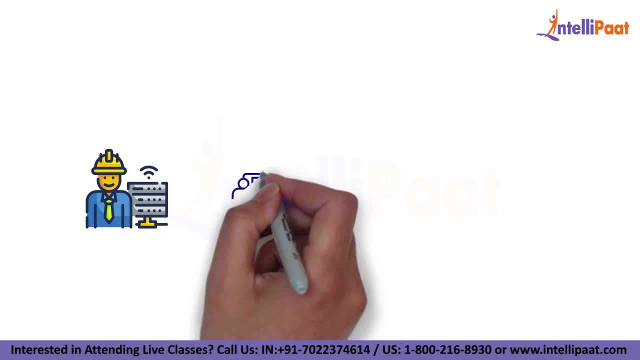 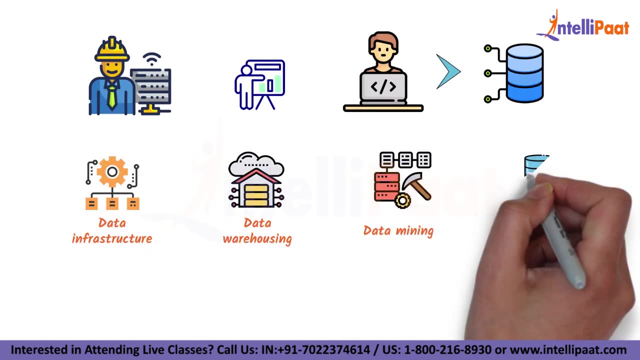 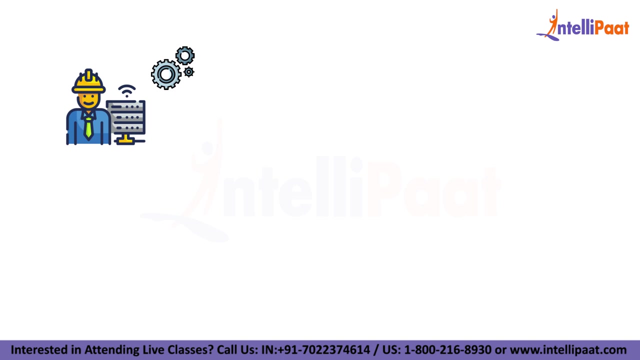 organization. Data engineering came to be described, a kind of software engineering that focused deeply on data, Data infrastructure, data warehousing, data mining, data modeling, data crunching and metadata management. Data engineers work in a variety of settings to build systems that collect, manage and convert raw data. 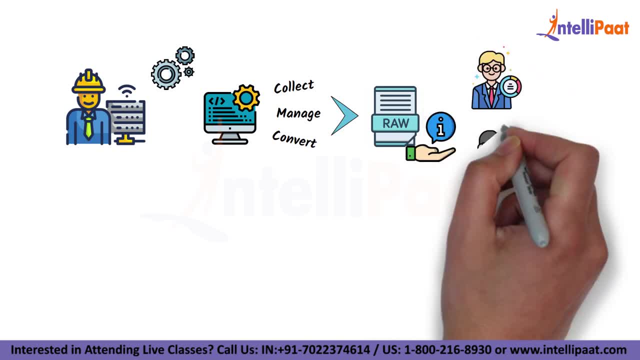 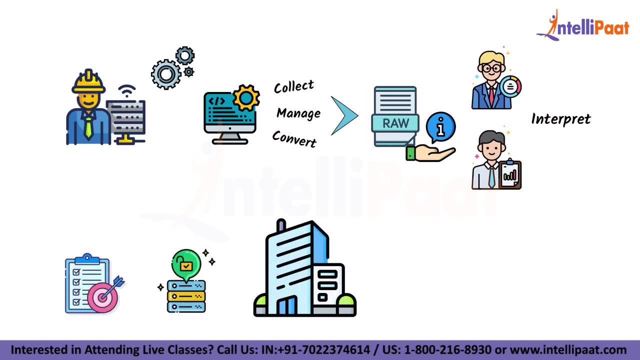 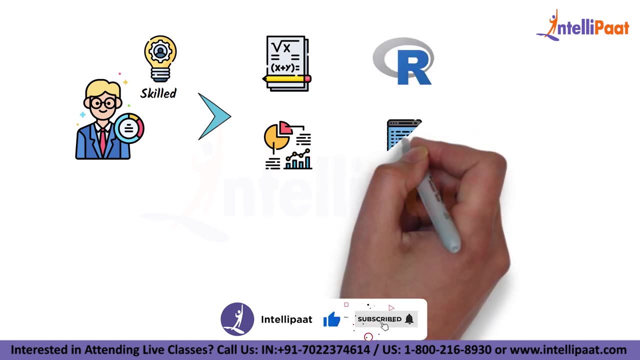 into usable for information for data scientists and business analysts to interpret. Their ultimate goal is to make data accessible so that organizations can use it to evaluate and optimize their performance. While data scientists are highly skilled in maths and statistics, R algorithms and machine learning techniques,